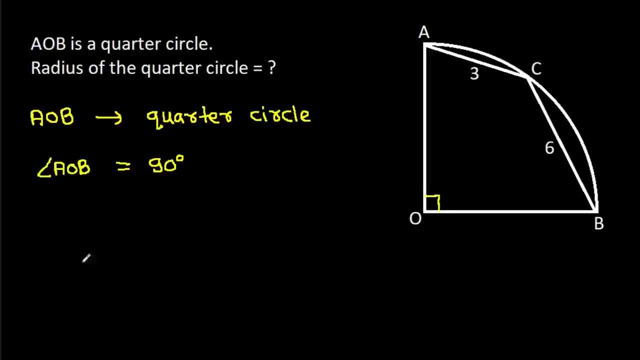 will be 90 degree, This angle, it will be 90 degree, This angle, it will be 90 degree. And angle around any point. it is 360 degree, So 8.0.. This angle is 90 degree, So this angle. 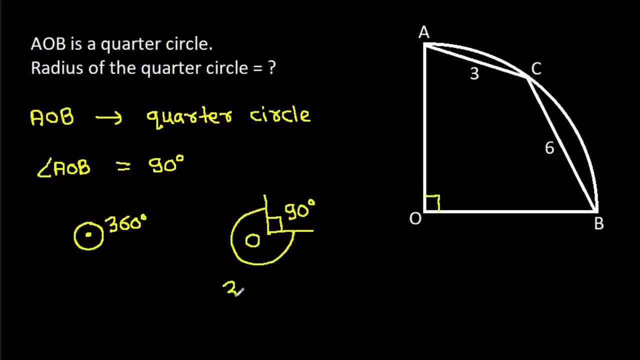 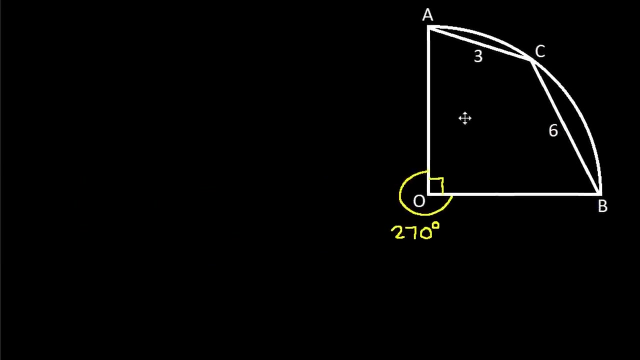 it will be 360 degree minus 90 degree. This angle, around any point, it is 360 degree, 90 degree. that will be 270 degree. This angle, it will be 270 degree and that will be 270 degree Now, in any circle, if any chord AB, if it is making an angle. 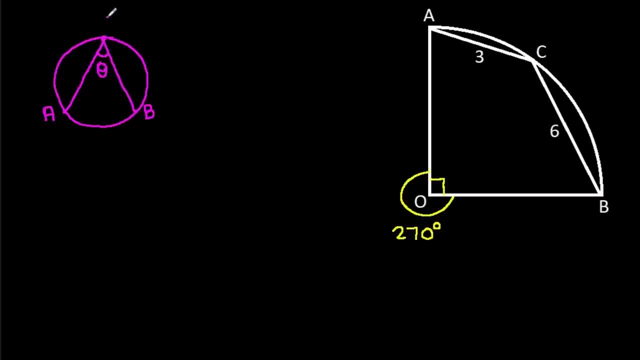 of theta on the circle. suppose this point is C, Then at the center, suppose O, it will make an angle up to theta And also it is AB, And if theta is greater than 90 degree, if this angle is theta, then at the center, O. 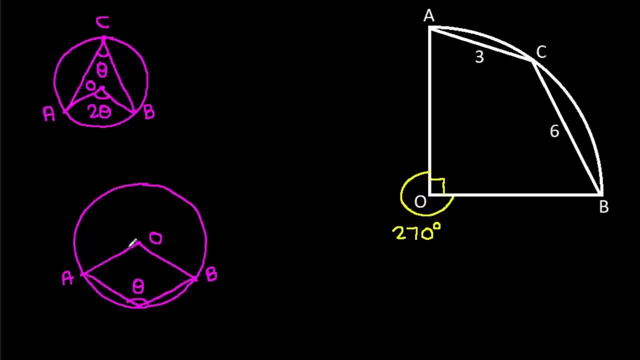 this angle it will be 2 theta. So here, if we complete the circle, then AB- it is making an angle of theta, Then AB it is making an angle of theta, Then AB it is making an angle of theta. 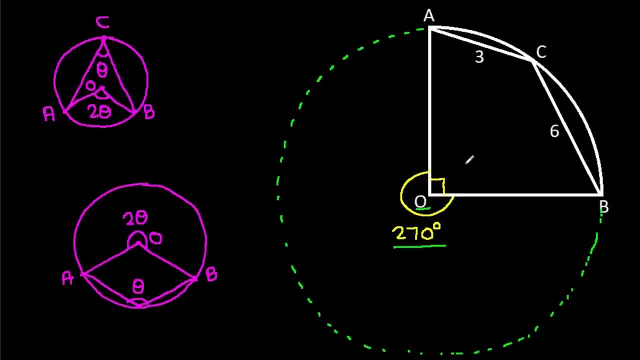 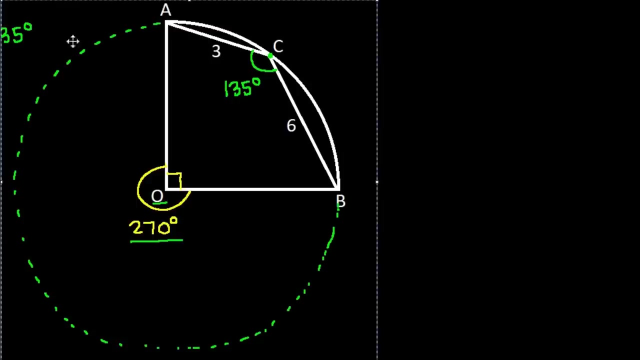 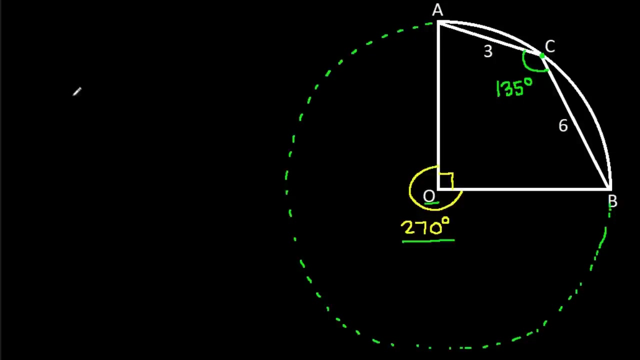 270 degree at the center. so at point C, this angle it will be 270 degree over 2, that will be 135 degree. this angle, it will be 135 degree. and now we know that AOB it is. 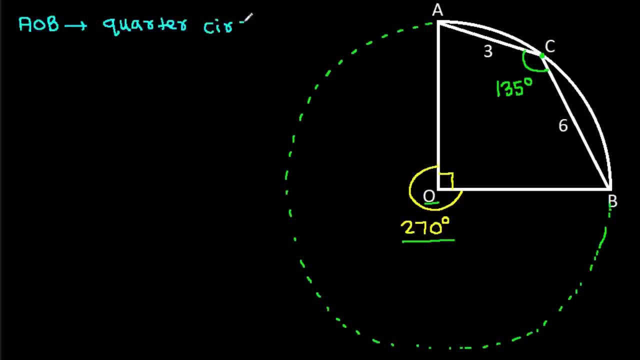 a quarter circle, Then we will know that this is a quarter equal to this angle. Suppose AO is R, Then we know that AO is R and that means AO will be equal to BO. that means AO-it will be equal to BO. that will be radius. suppose R, AO is R and BO is R, and if we join AB. 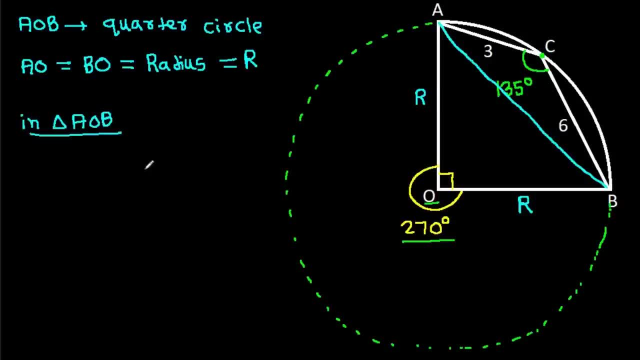 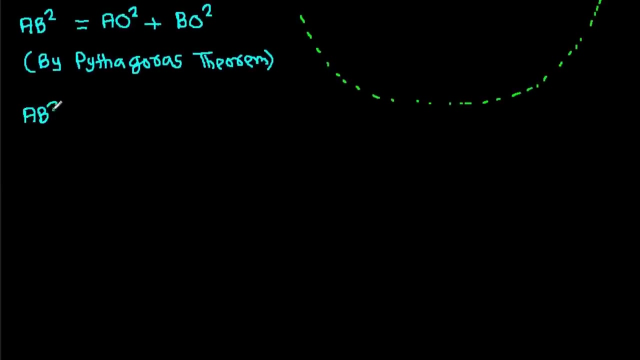 angle AOB it is AOB, AO is R, BO is R and this angle is 90 degree. So AB square it will be AO square plus BO square by Pythagoras theorem And AB square it is equal to. AO is R. 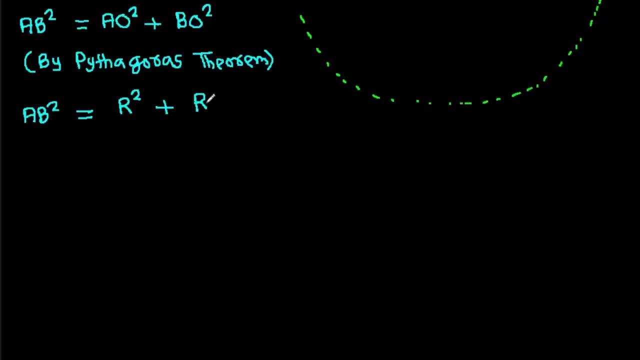 square plus BO is R And AB square. it is 2R square. So AB it will be root under 2R square. That will be root 2 times R. So we get AB. it is root 2 times R. 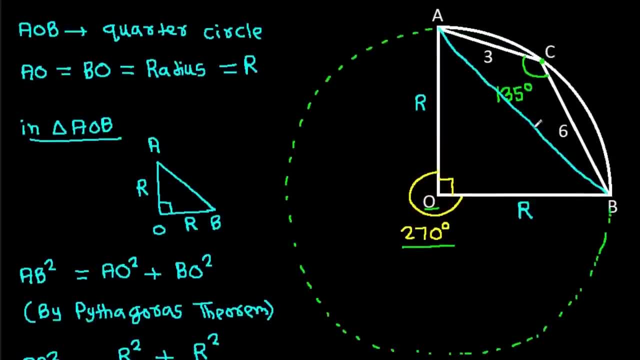 And this angle AB square, it is 2R square. So AO is 8, so AO is 2, OH is 8.. And it will be root under 3R square plus BO times RO. that will be 4R. it will be 4 times. 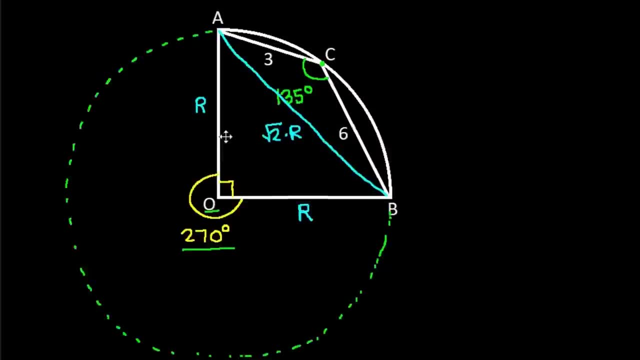 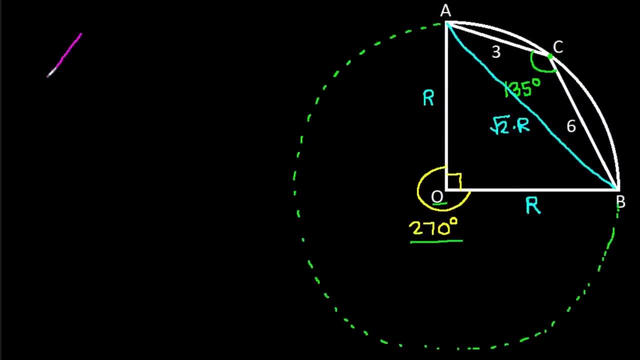 RO and right angle. This angle says: whatever angle you have in the video, whatever your angle users select. for this, all the indicators should be a single entry: elevation. All right, Now something else you should know: A, B, C. 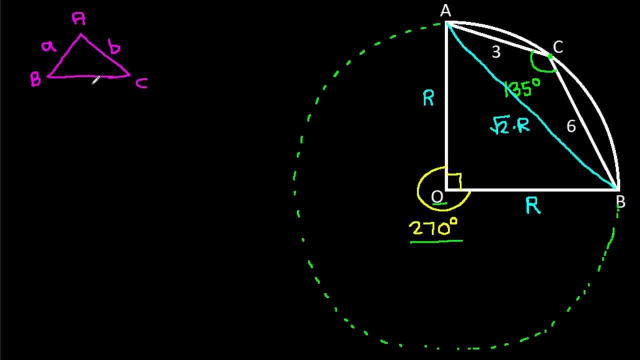 Now in any internal angle A, B, C, If A, B, C, A, B, C is a, ac is b and bc is c and this angle is theta, then c square it will be a square minus b, square minus 2ab, cos theta. so here inter angle a, b, c, it is a, b, c, ac is. 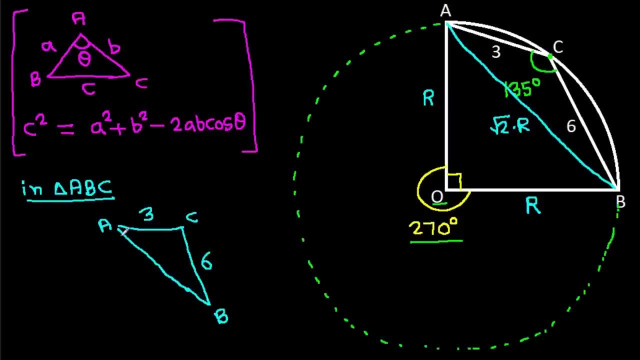 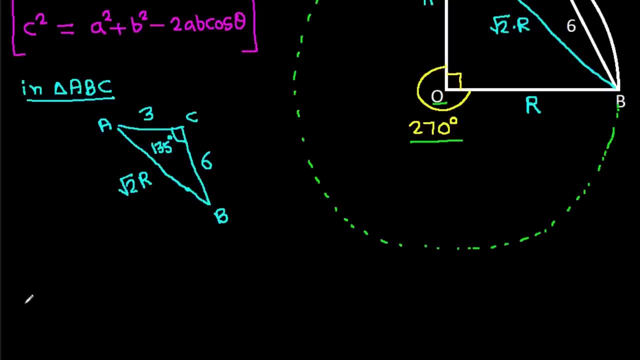 theta bc is 6 and ab it is root 2 r and this angle is 135 degree. so root 2 r square, it will be 3 square plus 6 square minus 2, times 3.. times 3. times 3.. 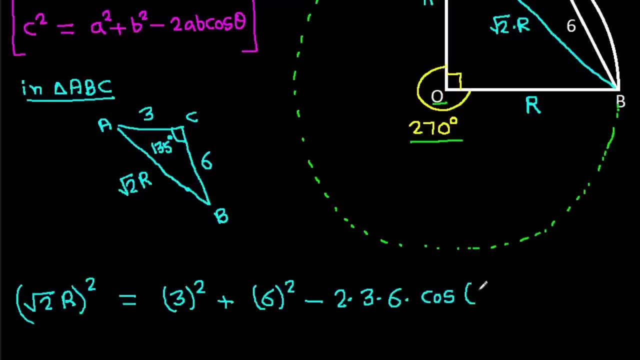 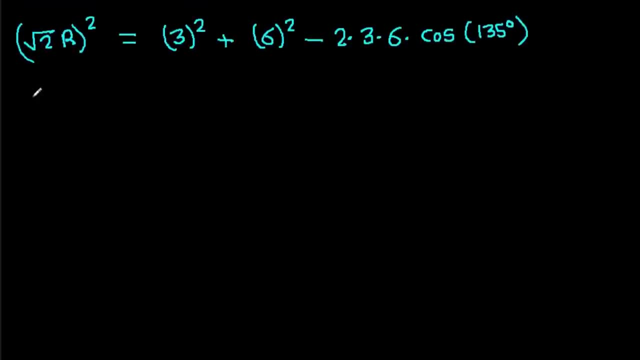 times 6 times cos 135 degree and it will be 2 r square is equal to 9 plus 36 minus and 6 times 6 will be 36 times and cos 135 degree. it is minus 1 over root 2 and 2 r square, it is 45. 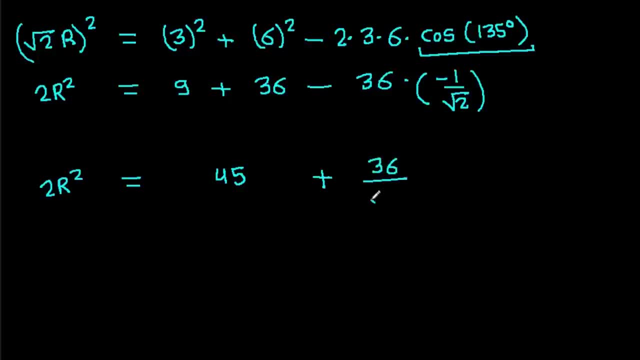 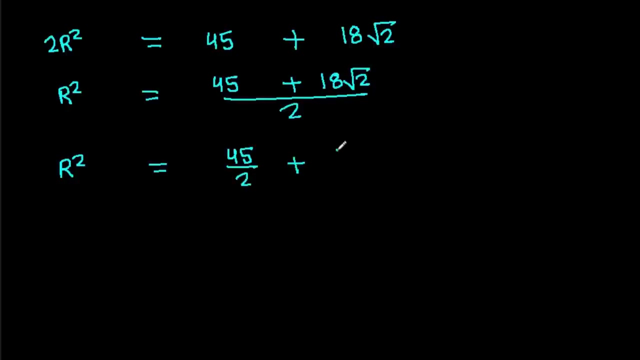 plus 36 over root 2, so 2 r square it is 45 plus and 36 over root 2, it will be 18 root 2, so r square it will be 45 plus 18 root 2 over 2 and r square it is 45 over 2 plus 9 root 2.